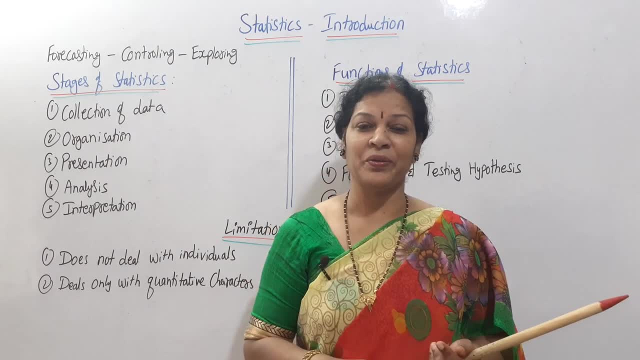 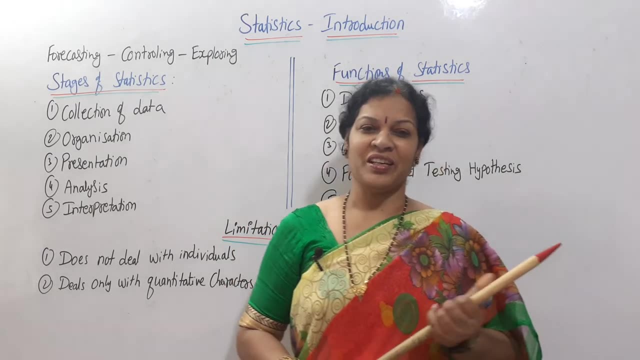 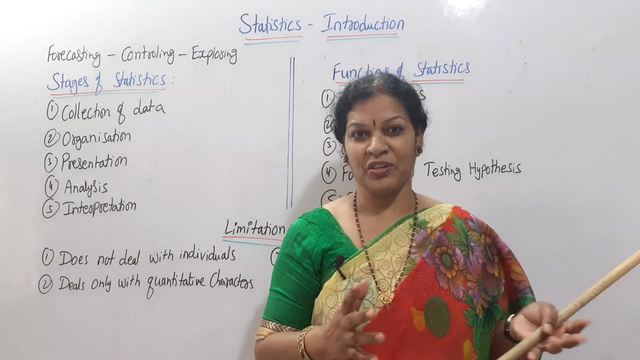 friends And they have to work out very clearly, wonderfully, without any hesitation. Remove that fear. Okay, now coming to statistics. What is the statistics? Statistics is a part of mathematics. you can say Generally the statistics is using by the sociologists and also social purpose. 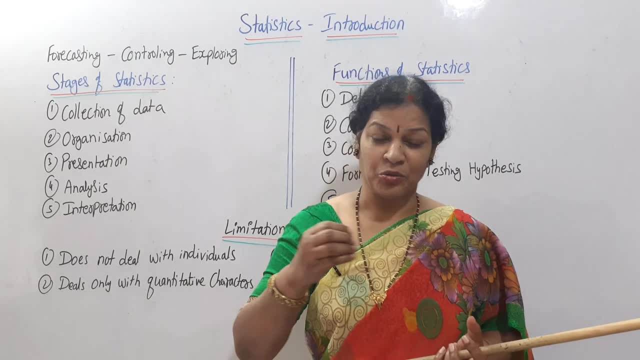 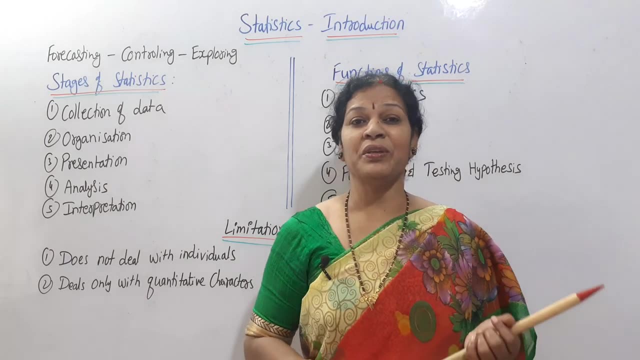 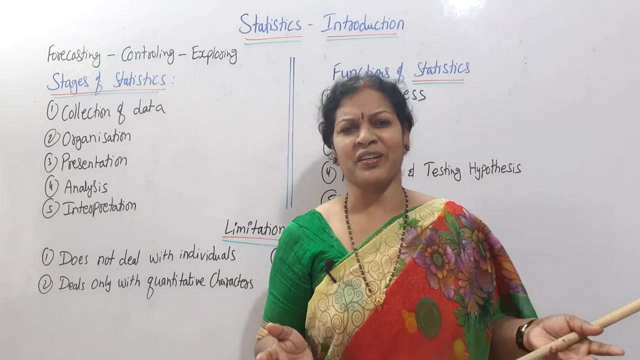 political purpose and sub data, And it is also for the economics point of view And also from the science point of view. We can use this statistics, especially business people. They use statistics a lot. Statistics means what? collection of data properly and presenting the data in a proper way to everybody. 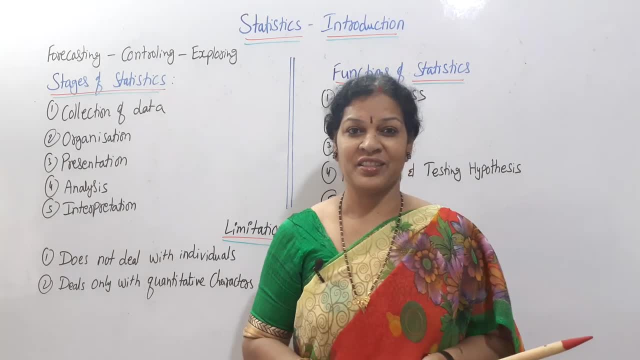 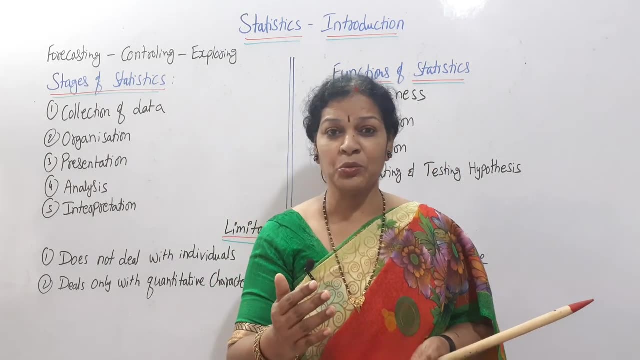 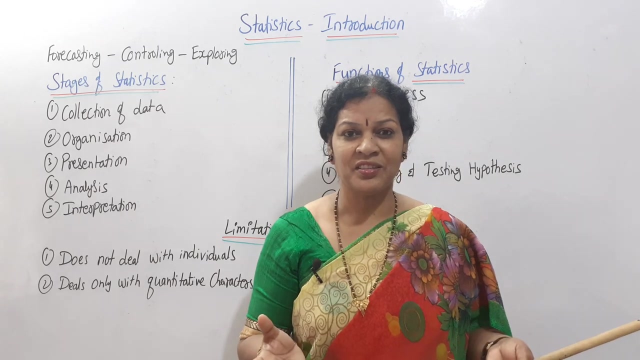 so that anyone can understand what it is. A layman, suppose, sitting in front of you some data you have collected and you are presenting in such a way through graphs, through bar diagrams, through pictures, through tables. That's it. That's the statistics Anyone can understand. You can make them to understand. 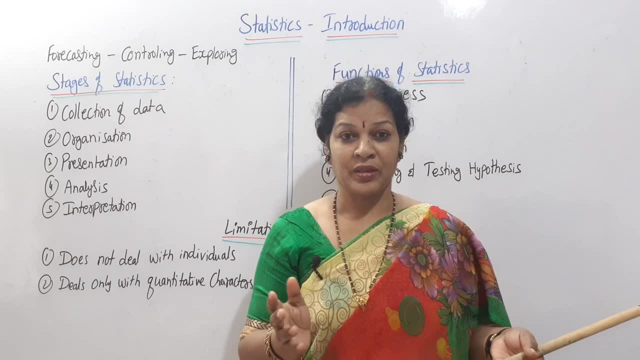 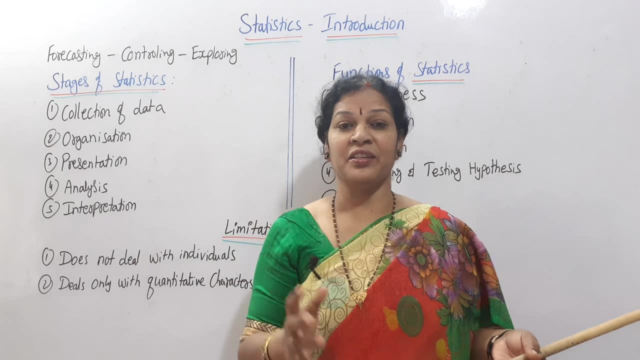 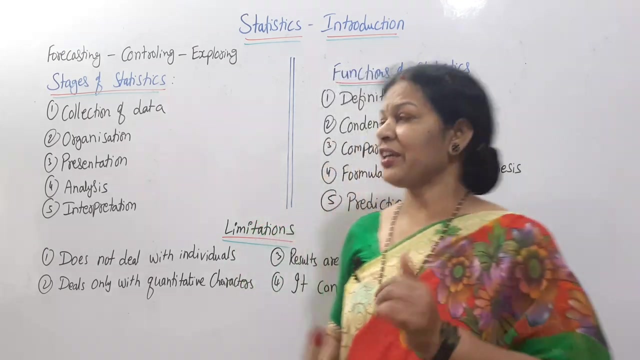 also Means the presentation Collected data, whatever is required to the other party: present it in such a way that everyone can understand it. So there are many uses of statistics. The main object, the main object of the statistics, is that: forecasting, controlling and exploring. 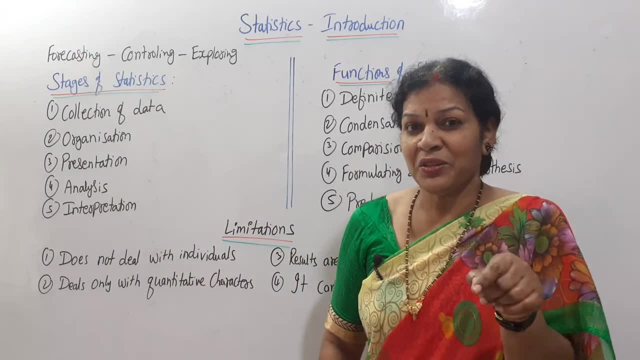 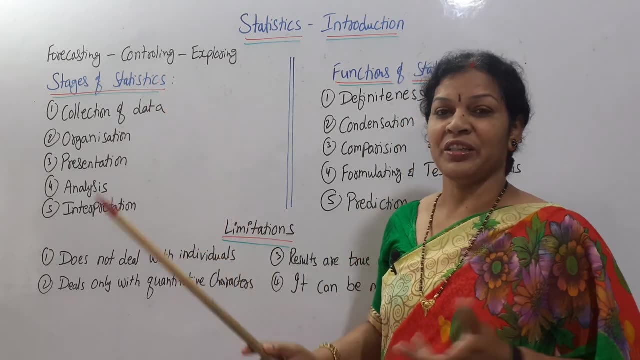 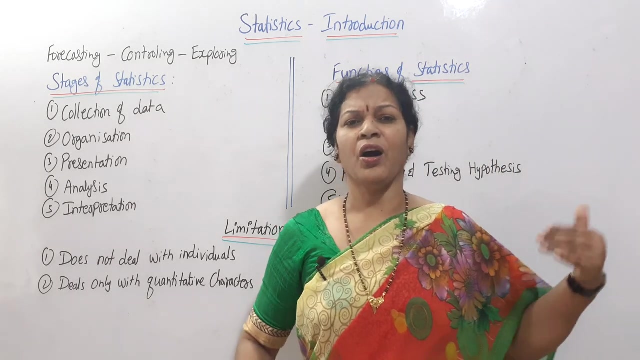 Forecasting future, what's going to happen. Once if you know that what's going to happen in future, then controlling is easy. Once if you control it automatically, it comes to the exploring. So these are the main objects of statistics. Now, what is the? what are the stages of statistics? How do we start the statistics? There are different. 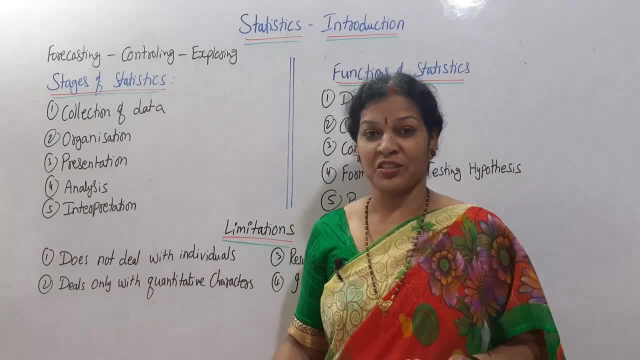 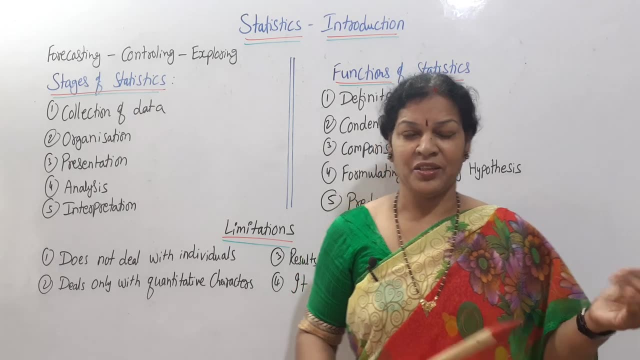 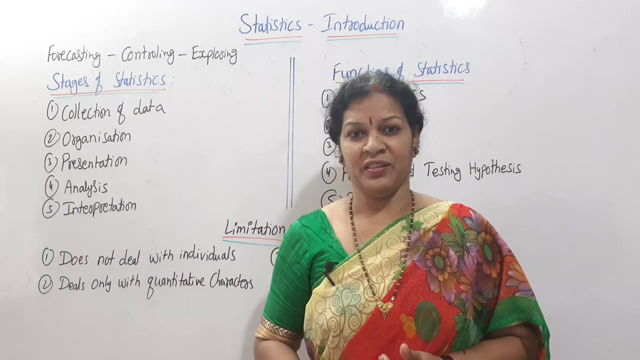 stages. Total stages are five stages, Step by step or stage wise. you have to identify, you have to know what is statistics. Second stage is that collection of data, Statistics directly. we don't work out problems. First of all we have to collect the data. This is much useful, even for the research scholars. 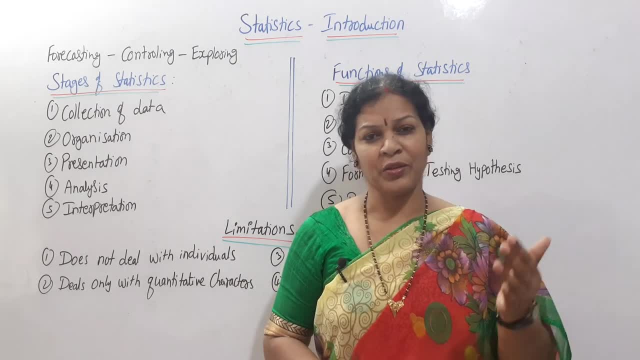 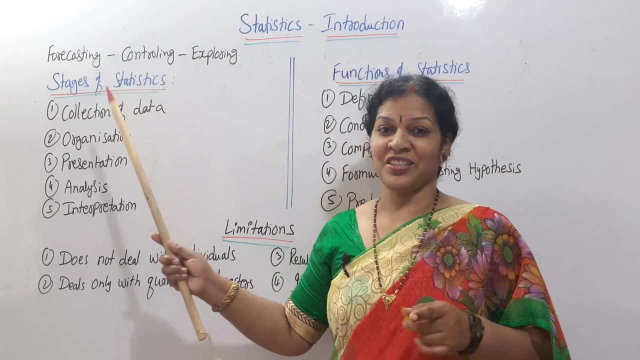 also When I have done my PhD at MPhil in those days also, first collection of data, then after the presentation, analysis and interpretation, like all these stages I have gone through. So that is why I am saying it is much useful, even for the research scholars. 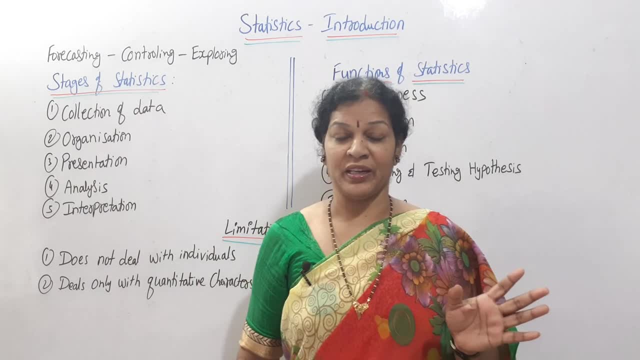 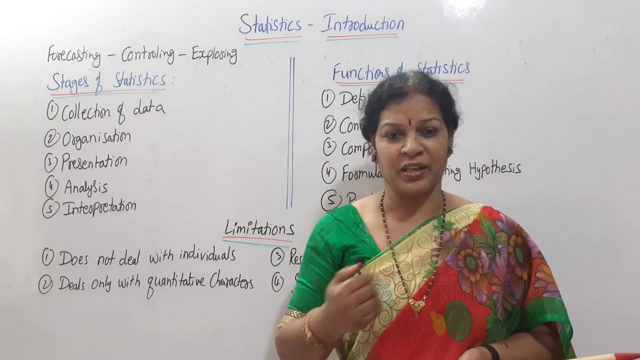 also, First, what we are going to do: Collecting the proper data. Collect the data. What kind of data, Whatever is required. Suppose I am doing research, I need some data So that I am going to collect And say: country, wise state, wise district. 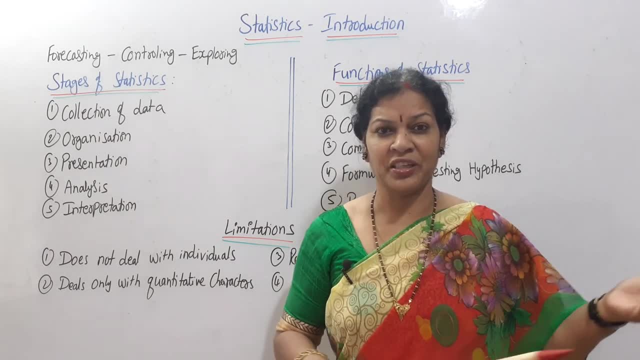 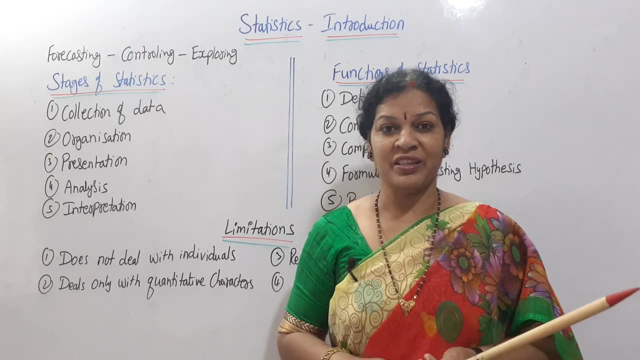 wise. some data is required: Population- they are counting it. Income of the people: they are counting it. And how many students are there in the school, How many boys are there, How many girls are there, Their marks, their score and income of particular company Income. 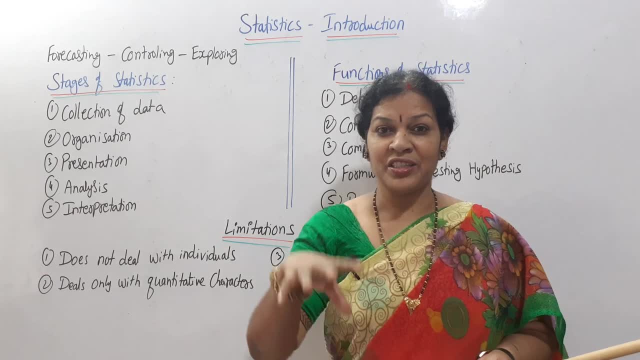 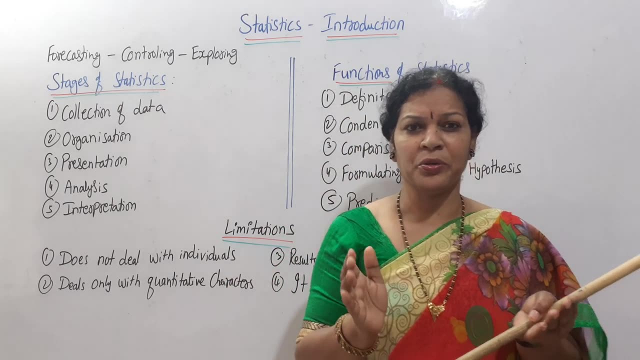 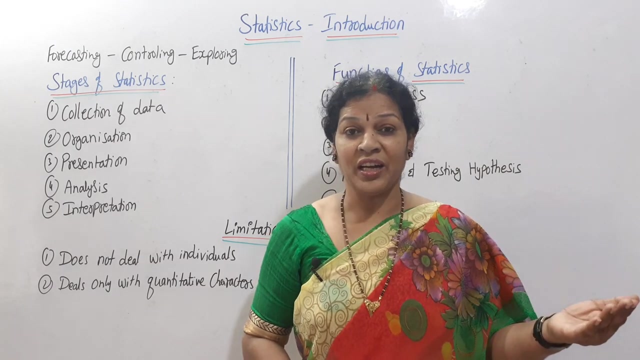 of particular group, So like father's age, son's age, So any kind of data, something we have decided that this we wanted to find out, This data we wanted to collect, That collection of data is important. How do you want to collect the data Through a format? 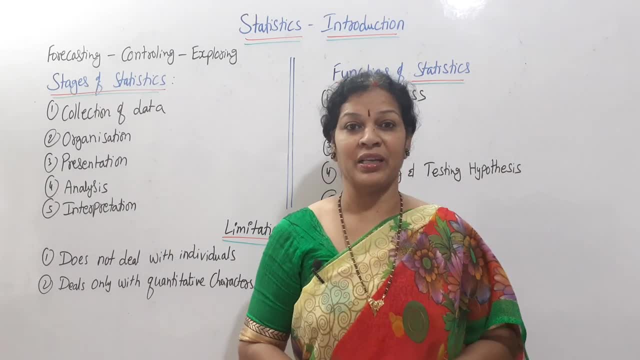 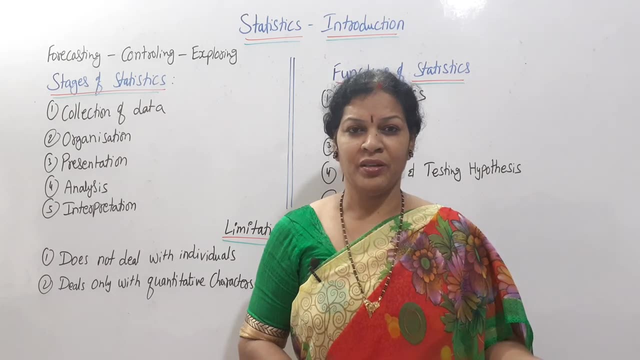 Through a format, something is prepared. then, according to that, you can go and collect the data. There are many ways: Personal interview, directly meeting the people, or through a phone, phone call, through a mail. In any way, you have to collect the data Once the collection. 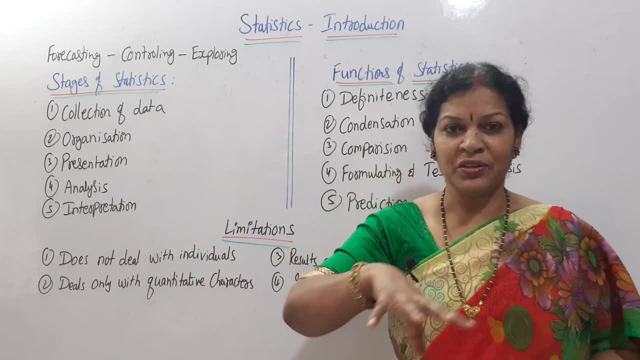 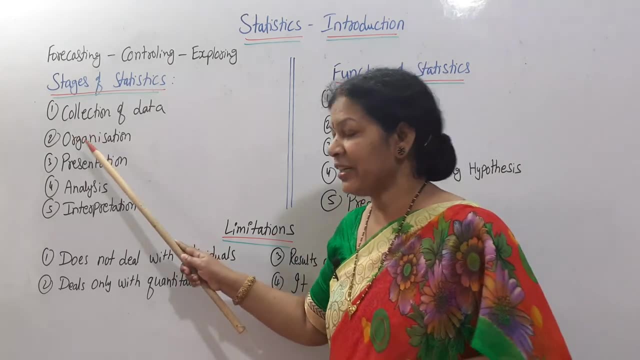 of data is over, next step comes to organization. So this everything is organizing in a proper way. Data is collected, Where do you put, Where do you keep, How do you want to proceed? it That is, we call it as a organization. Once organization is over, then presentation. 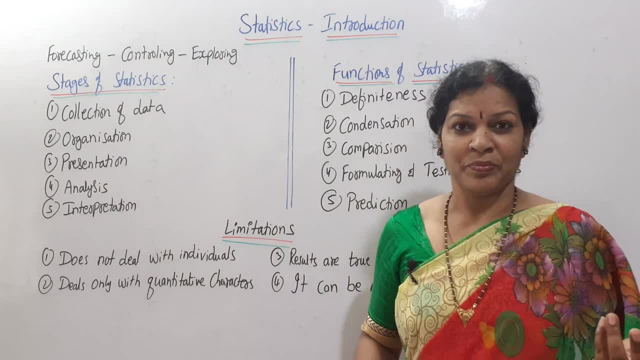 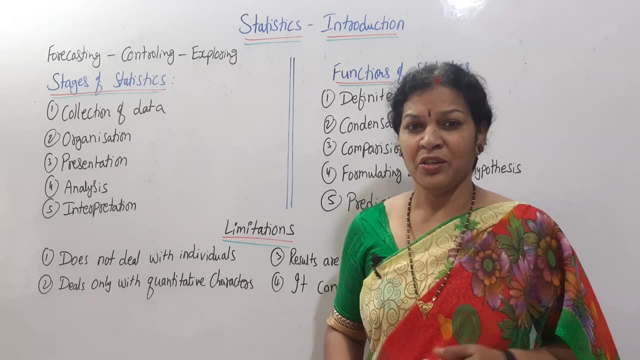 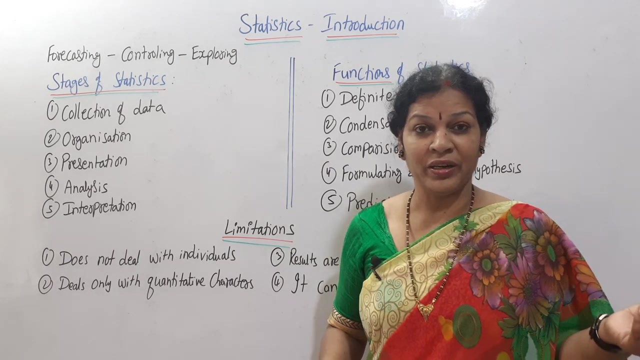 I want to present this data. How do I present it? In which way I wanted to present it. Should I present it in graphs? Should I present it through a histogram? Should I present it through tables? Should I present it through any formulas? Should I calculate anything required? So that's we. 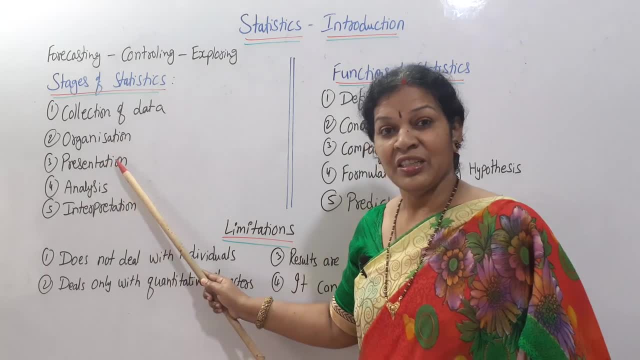 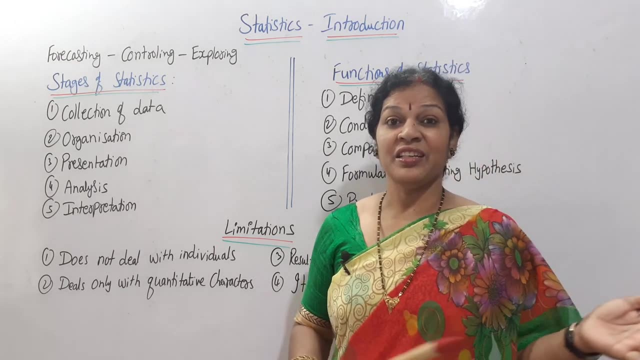 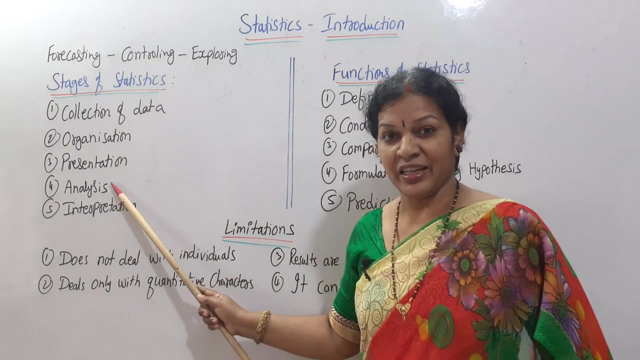 say it as a presentation. That presentation is interlinked with analysis. Analysis means you are going in depth, analyzing the data stage wise. How do you want to present? Different ways are there? So how do you want to present? That is called as analysis? Then, after that, 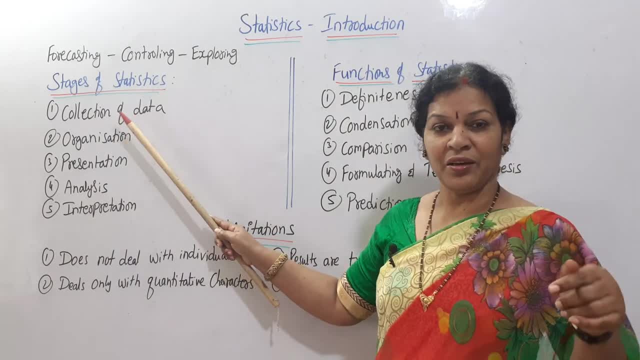 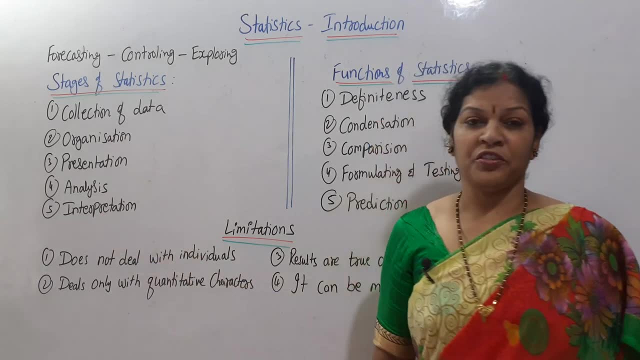 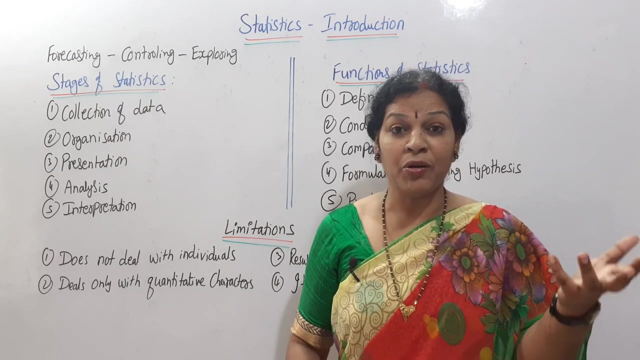 there is a complete interpretation. Okay, we have collected the data. organizing is over, presentation analysis: everything is over. Lastly, it comes to the interpretation. What is this interpretation? Interpretation means we are giving explanation, We are giving explanation about what I have done, What we have done, So that explanation we call it. 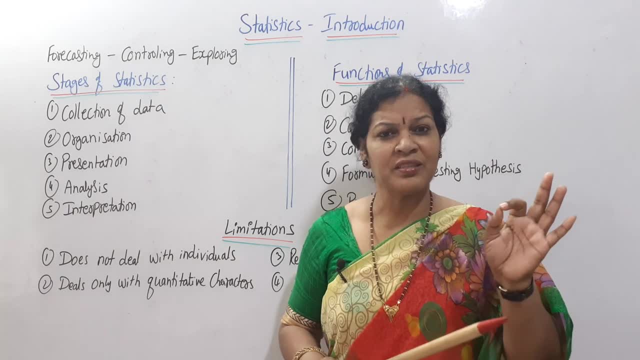 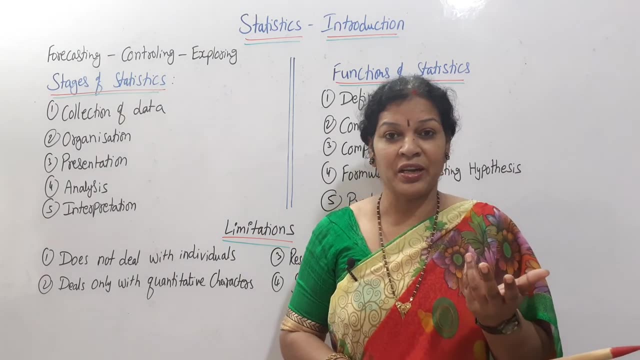 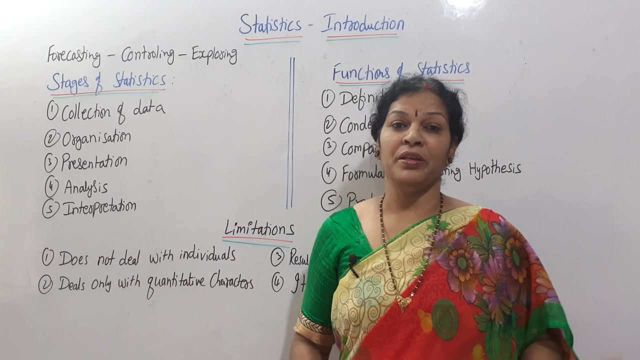 as an interpretation. Interpretation should be in a simple and easy language so that it is clear. A layman comes to you and if he wants to understand what it is, he must be in a position to understand. In that way, interpretation should be Interpretation. everybody cannot. 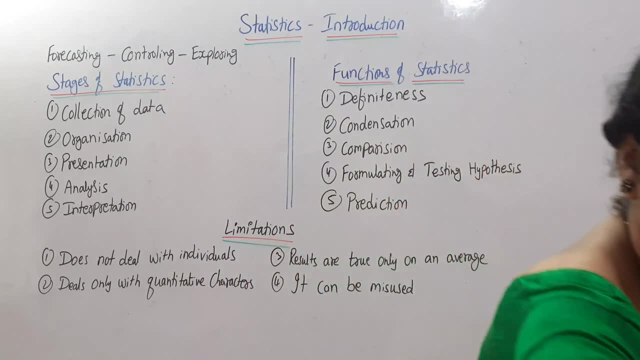 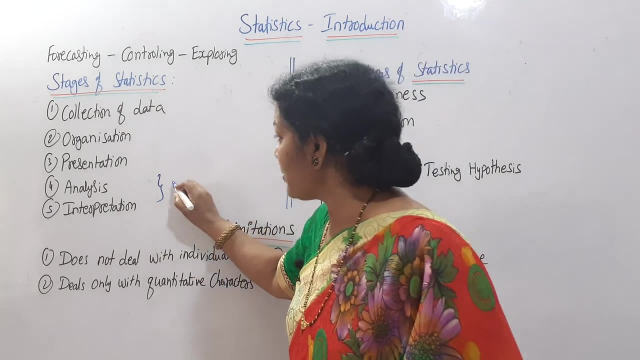 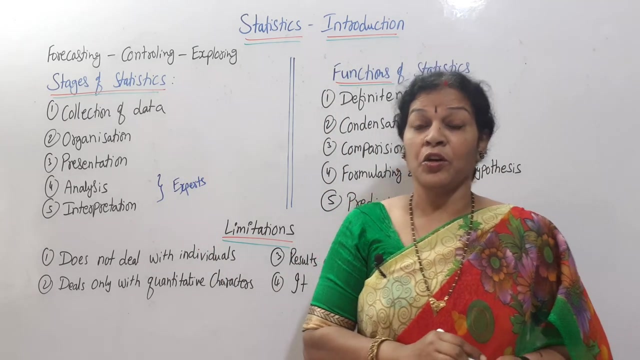 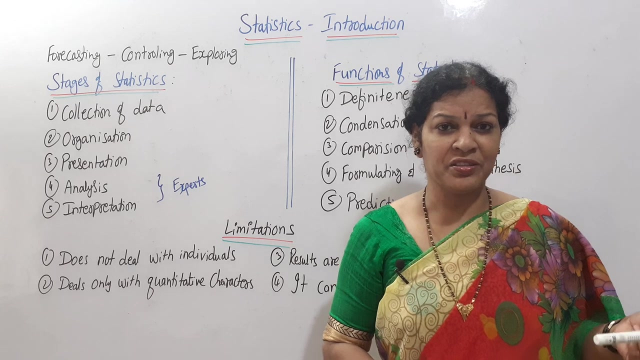 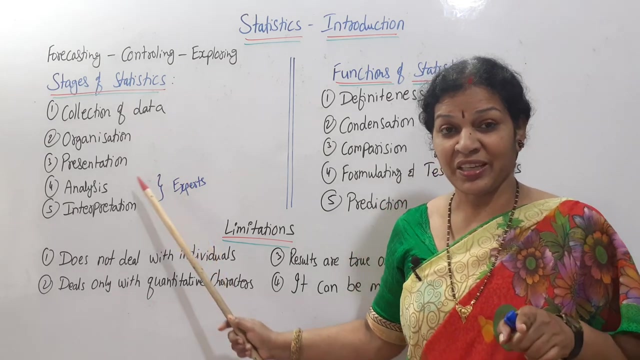 do Even analysis also: Analysis and interpretation. Analysis, interpretation- both of these can be done by the experts, only Who have good knowledge about This statistics. Only those people- experts especially- who are well versed in statistics and who have done MSC statistics or BSC statistics gone depth, Those experts can go for this analysis. 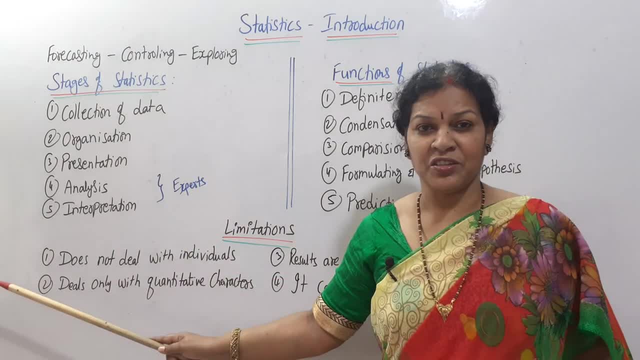 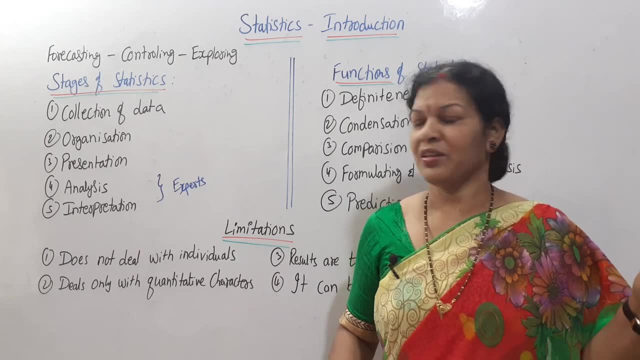 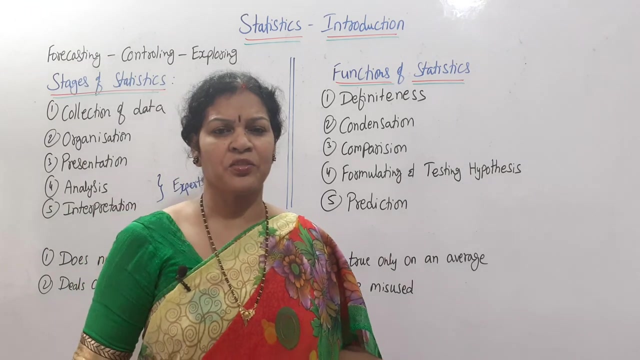 and also interpretation. Okay, so these are the five stages. Once interpretation is over means statistics, that particular part, whatever object is there that is over. So that is about stages of analysis. Next we will see functions of statistics, How the statistics going to work out. First, 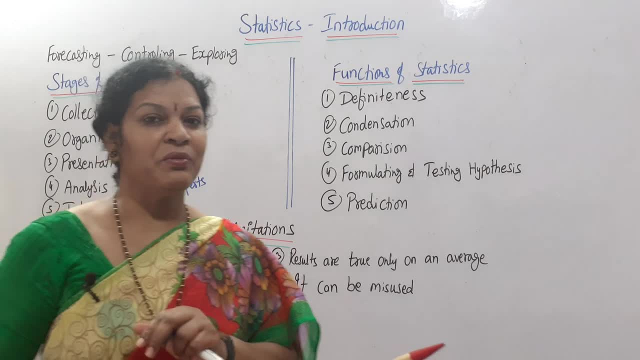 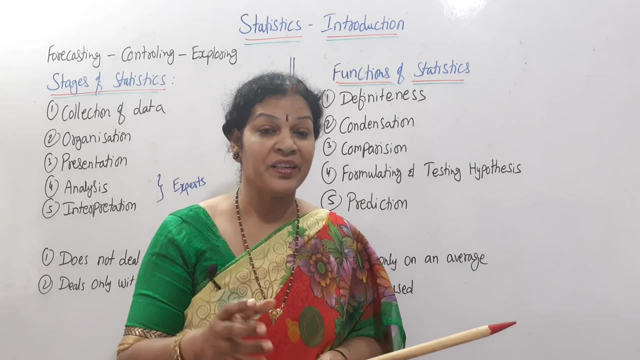 of all, main function is the definiteness Statistics. whenever we calculate something, whenever we present something, that accuracy, that 100% accuracy, you will find it. that definiteness you will find. You will not find any vague information. You will not find any. 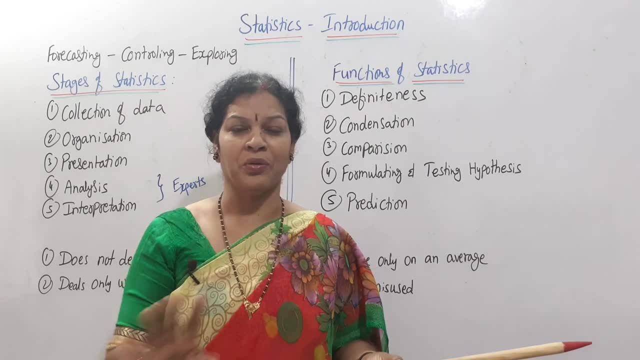 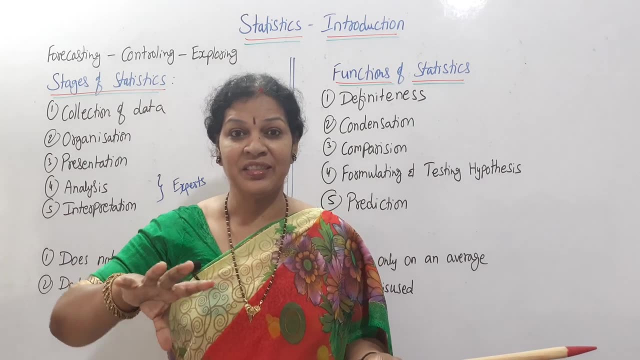 fictitious or some other information. No, Whatever we do, because we have calculated, we will find. Whatever we do, data through the data only. we are going for organizing and analyzing interpretation, all this thing. That is why definiteness is one of the main function. 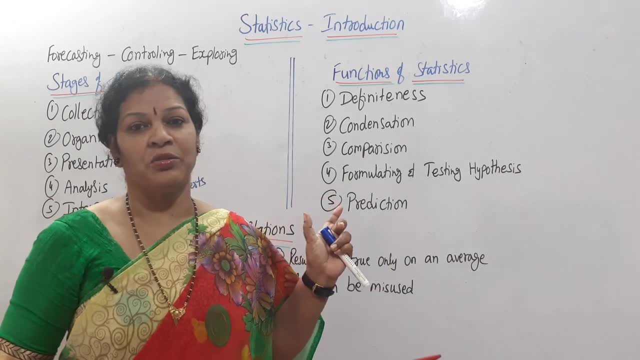 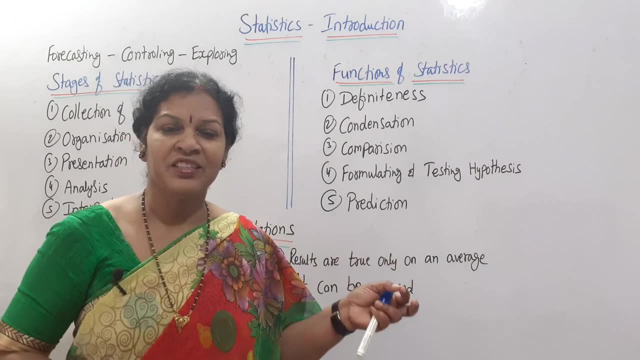 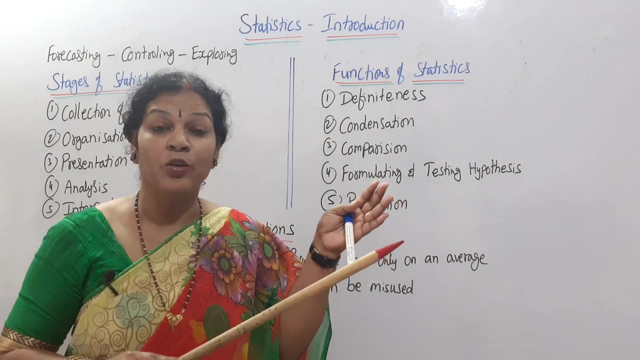 of statistics. Whatever we do, accuracy will find, In the same way, Condensation, the data. we do not present it simply. we will be condensing means we are minimizing it. We are minimizing and we are presenting the data in a systematic. 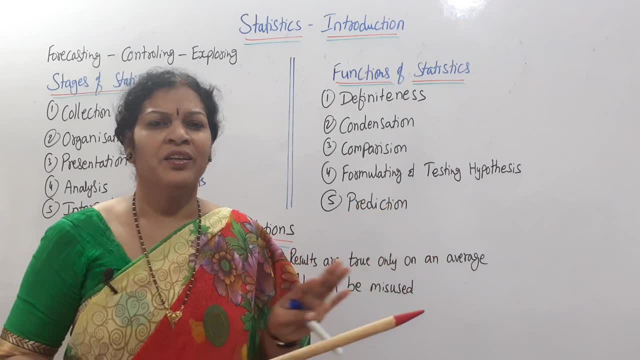 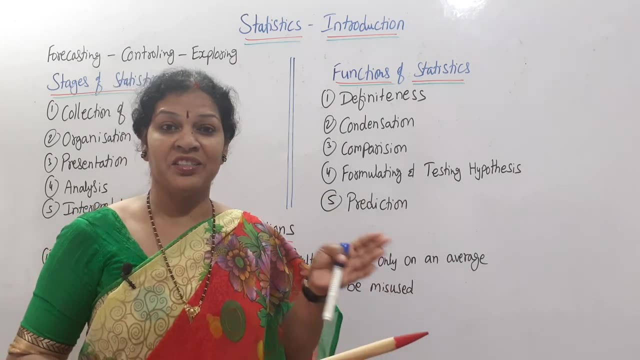 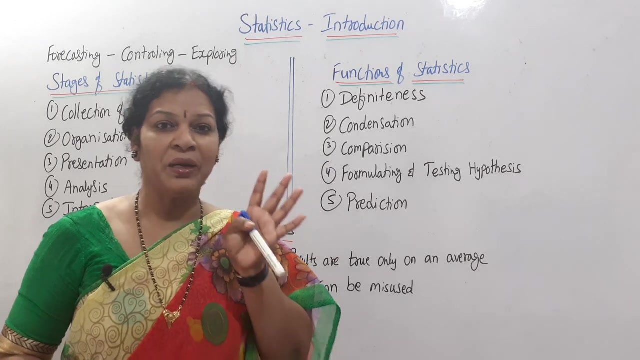 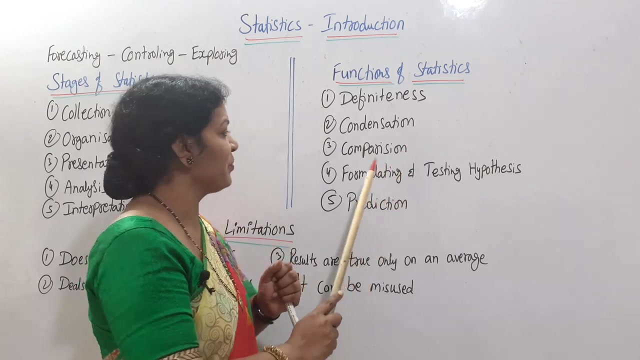 and lucid form. The sometime we 18 sound still not charged. And finally, we are minimizing what we have used To defini So that anyone can understand. So we are not making much struggle to others to understand. We are making it very easy. Condensed means, in shortcut, in a simple way, in a lucid manner. So in that way we are presenting the data. This is also one of the main function: Condensation Minimizing and in a lucid form. 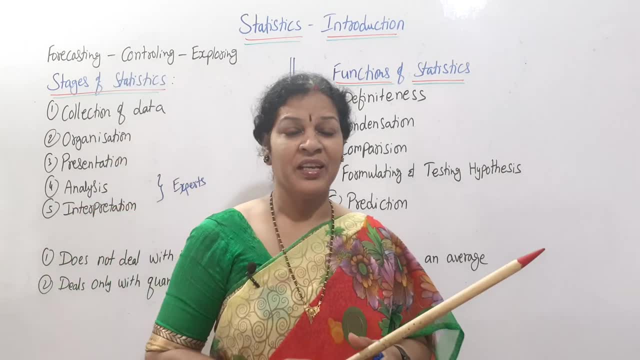 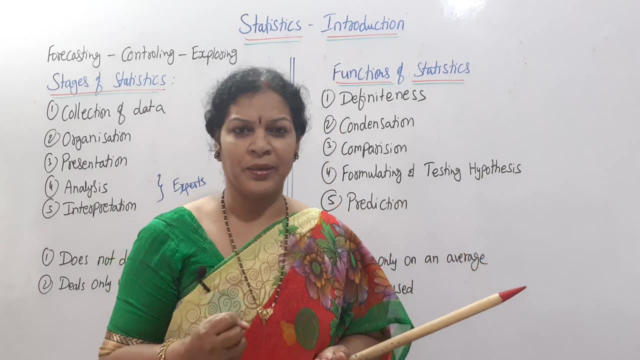 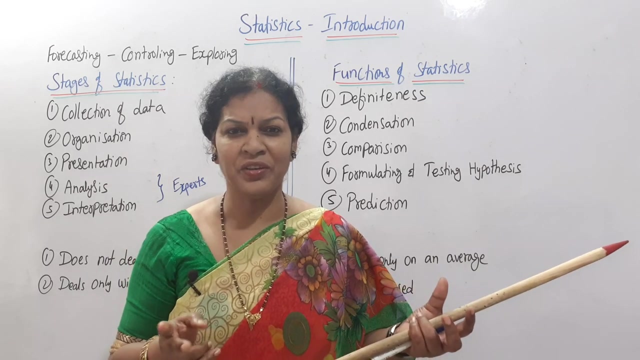 Next, comparison: Data is collected means the data is ready to compare with anything. This is also main function. Say, data of X company. I have collected. Data of Y company also collected. We can compare it. How is the performance of A, How is the performance of B? 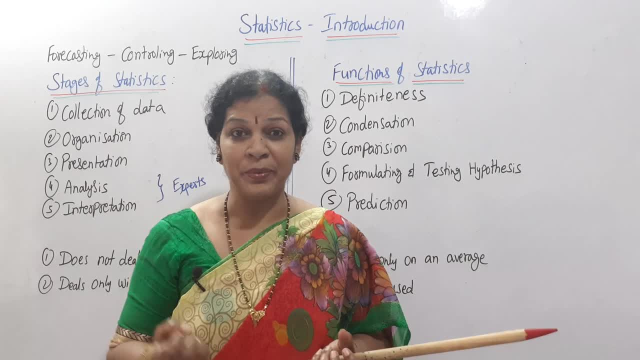 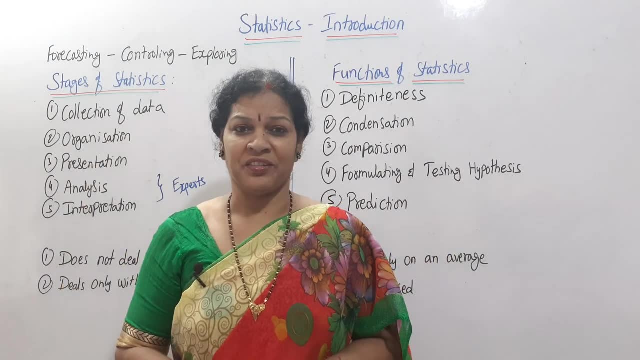 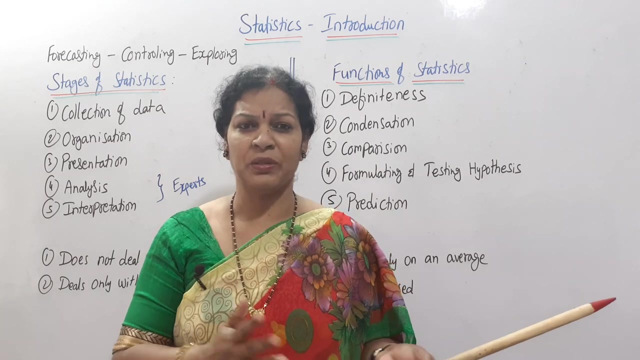 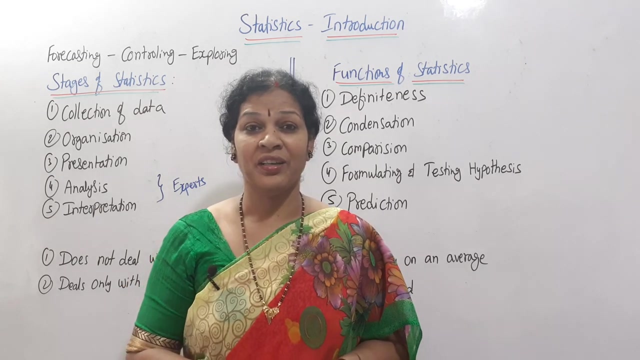 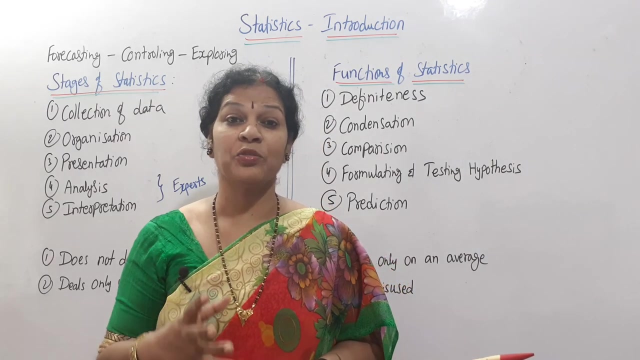 Production of A and B, Sales of A and B And growth of A and B, Profits of A and B. Like many areas of the world, Like many areas, we can compare it. Comparison is possible Between two companies. I said it can be possible with anything Between two states, between two districts, or two cities, two countries. you can go ahead, There is no limit at all for this statistics. You can go beyond imagination also, because that kind of scope is there for statistics. 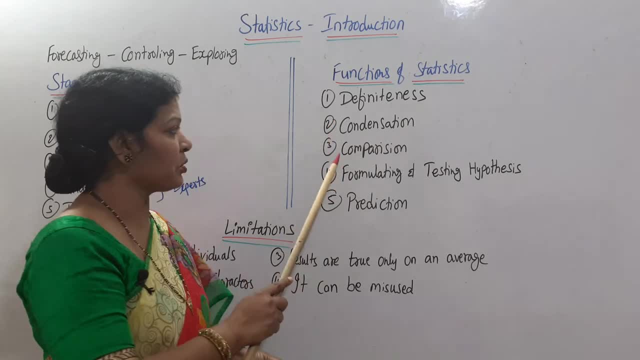 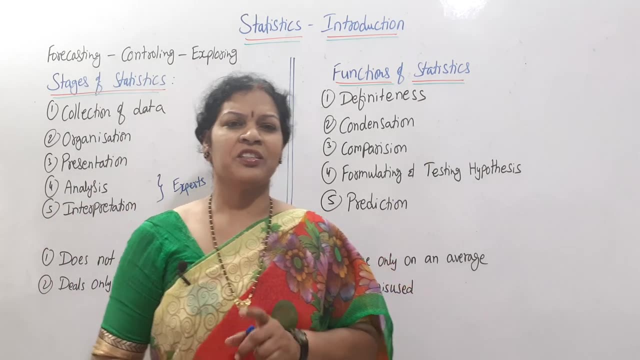 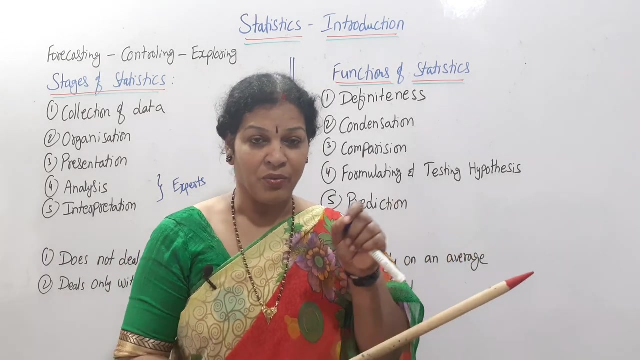 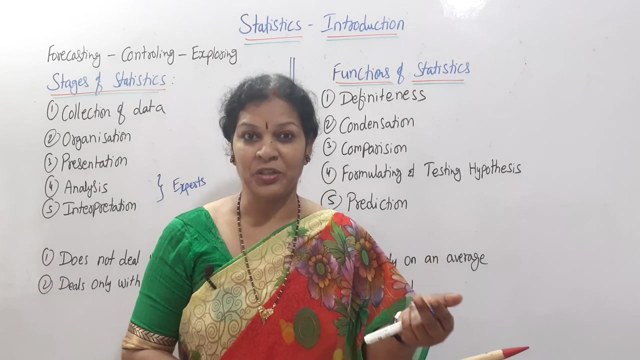 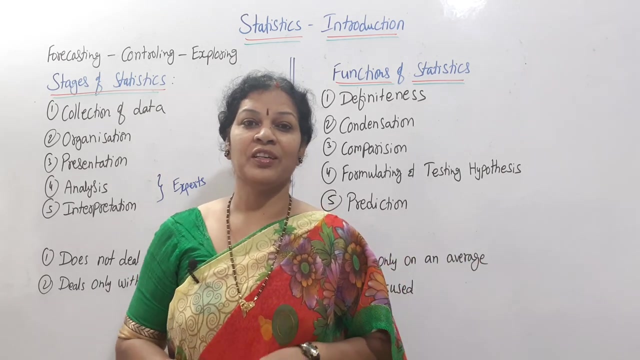 So second function is condensation. Third one is comparison- I spoke. And fourth one is formulating and testing hypothesis. Formulating and testing hypothesis, which can be done only by the experts, only This one. also. This shows whether whatever data we have collected is it correct or not. Is it signifying the exactly information, what you have collected, or not? So that is called as hypothesis, Constructing of hypothesis, Then after the testing of the hypothesis. So there are many tools in statistics. 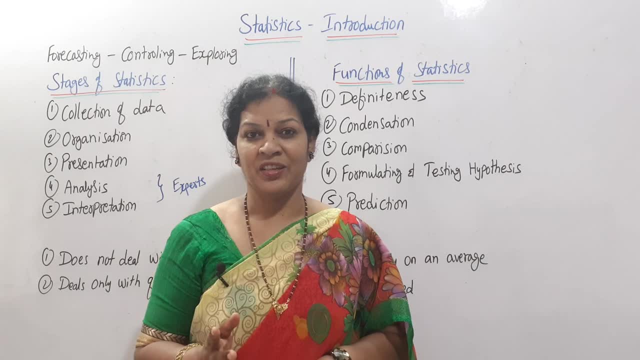 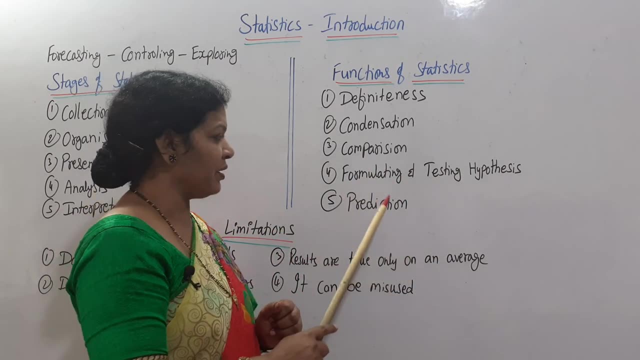 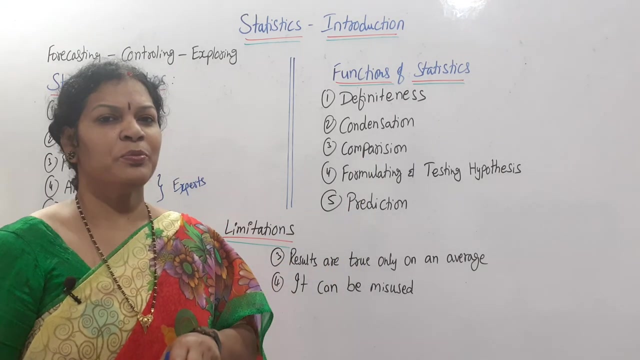 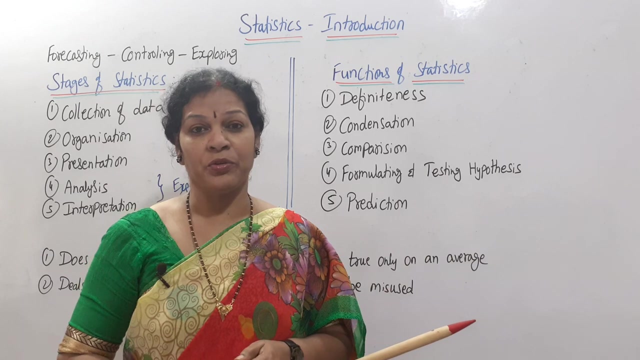 Especially Kikesware T-test, F-test, So that kind of tools we use for the hypothesis, Construction of hypothesis. So this is the fourth one, And in the coming classes you will come to know. Then important function is prediction. Statistics means we have collected the data, presenting the data At the same time we can predict, we can forecast what is going to happen in future. Say, we have collected the data For the last 10 years. sales are like this: 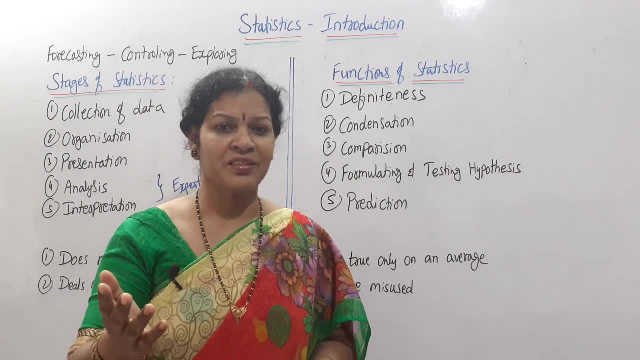 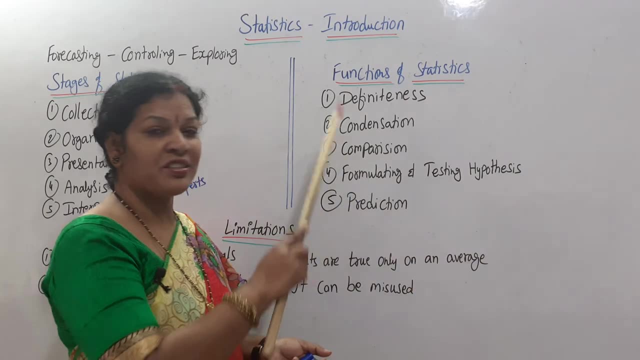 And what would be the sales in the next year? What would be the sales after 5 years? What would be the performance of the company after 5 years? Like this prediction also possible in statistics. So that is prediction. These are the main 5 functions of statistics. 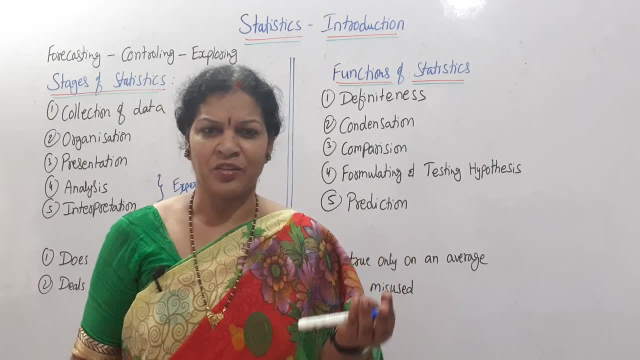 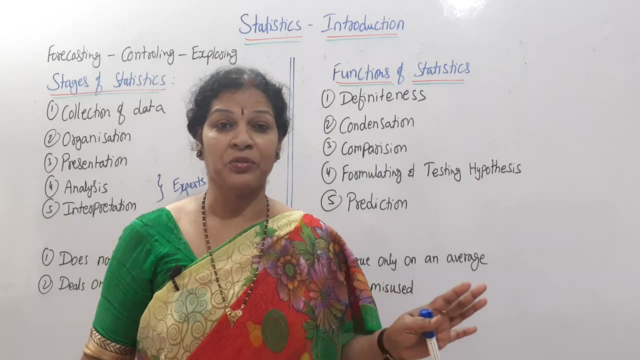 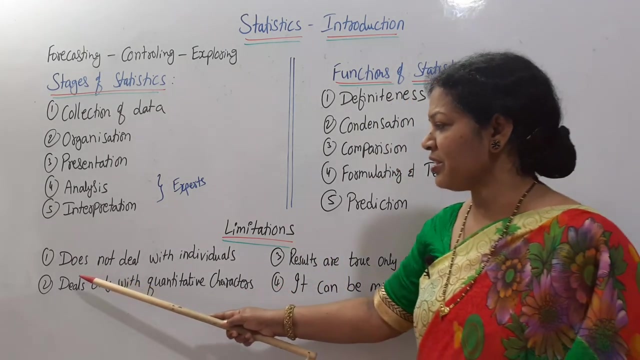 Yes, statistics is useful for everyone At their economics or business and mathematics point of view, and social Everyone they are using it, But still there are few limitations. What are those limitations? Just simple 4 limitations. First one is that does not deal with individuals. 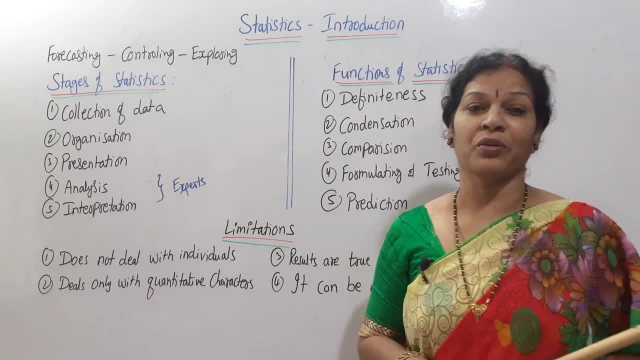 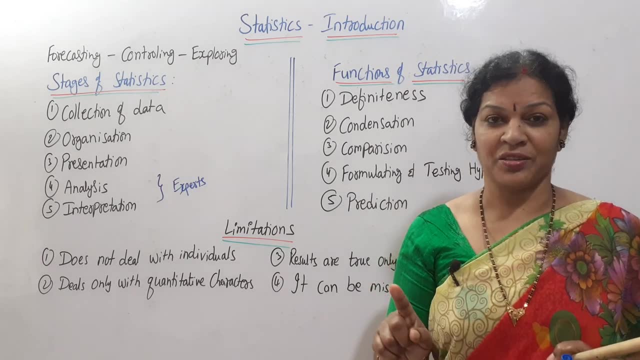 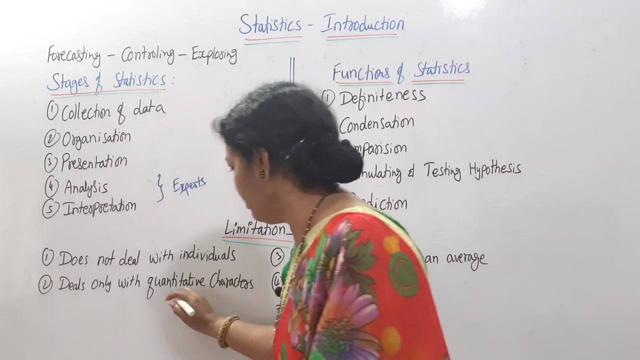 Statistics means group of information, Lots of information we focused. It's not focusing on the individual series, Individual item. it's not focusing. So this is one of the drawback. And next one is that it deals only with quantitative characters, Only quantitative Quality, No. 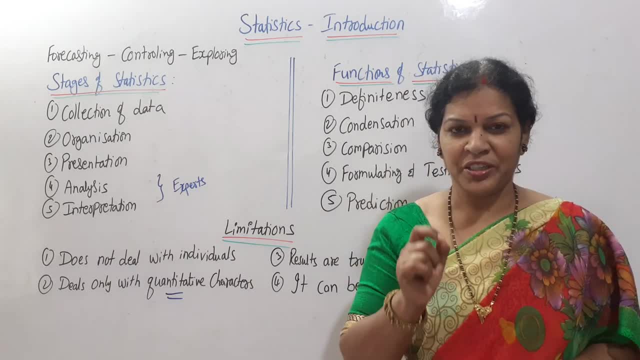 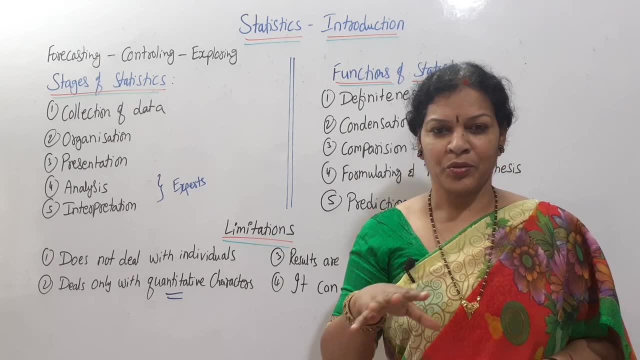 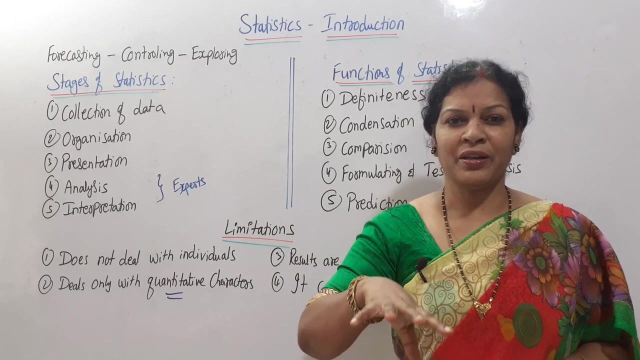 Not going to bother about the quality of the information, it's quantity only. we wanted to collect the data of 10,000 people, we want to collect the data of thousand people. so is it having the quality or not? is it possible? so are the people are universal, so that kind of 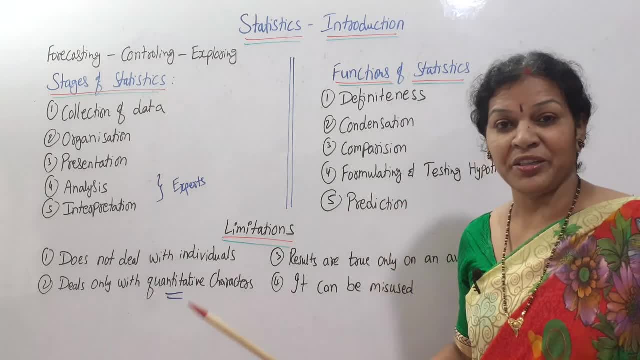 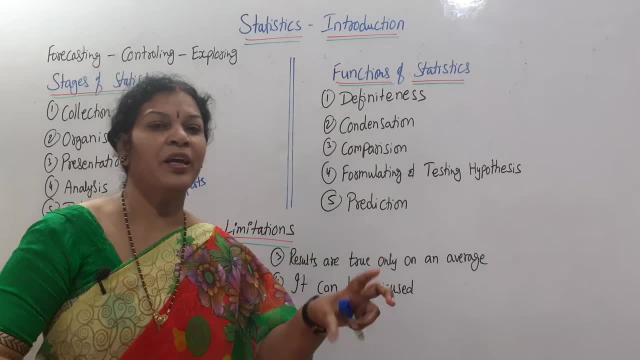 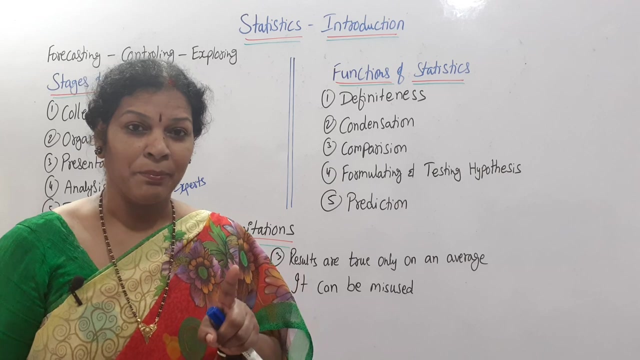 quality. we are not seeing. we are just focusing only on the quantitative data, only. next one: results are true only on an average. there are many tools, many techniques to calculate in statistics. many, very many items we can calculate, but only an average hundred percent sure. others may or may not be. 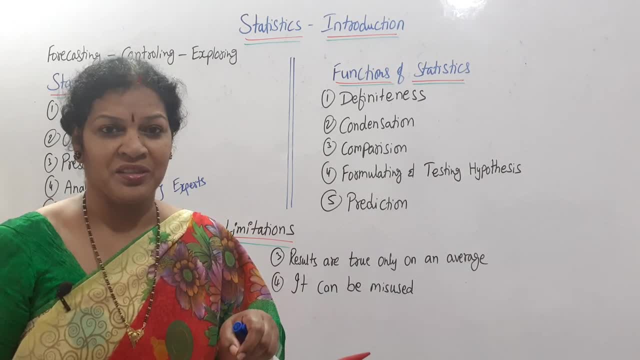 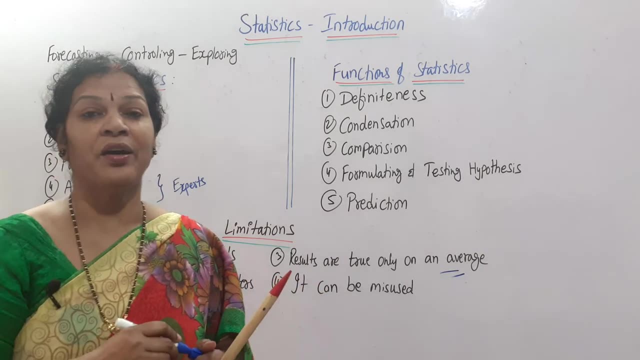 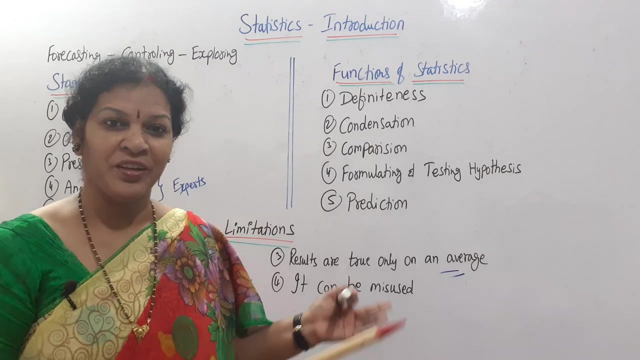 sure it is not there in other tools, but only only it is true in an average, only, only an average. so that is the calculation, only average. it is true- others there may be a lots of fluctuations, may not be hundred percent perfect, but only average is perfect. this is one of the drawback and 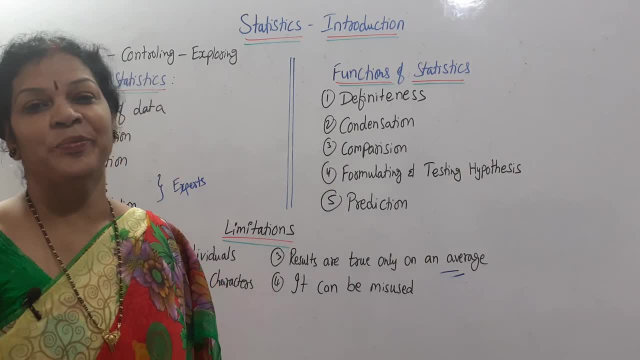 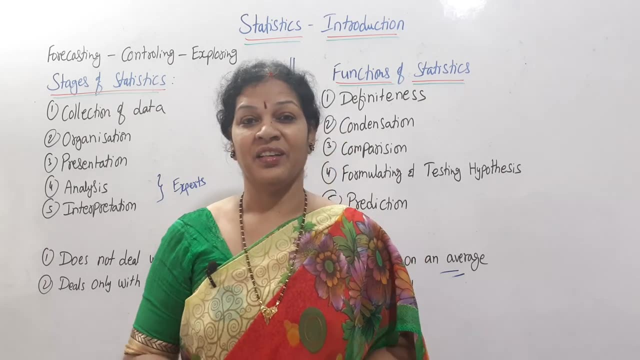 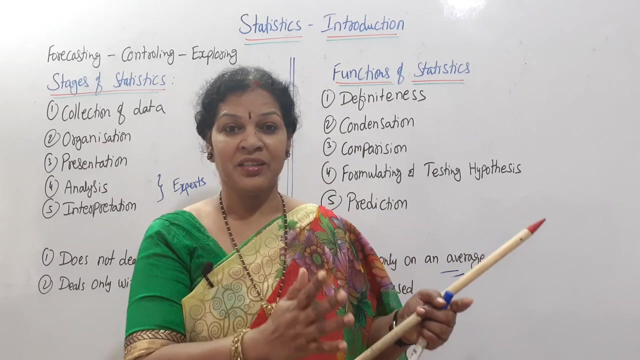 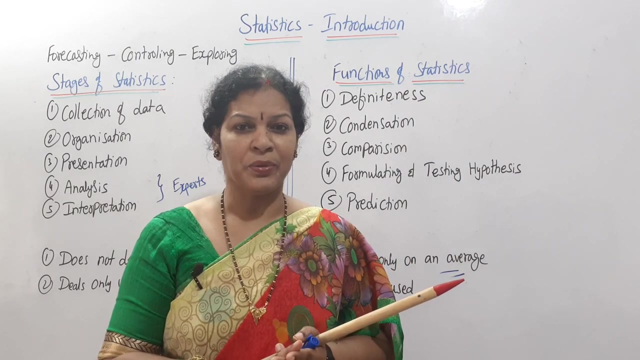 last one is that it can be misused easily. it can be misused easily. data is collected, but presentation is doing by somebody and analysis is doing by somebody, and also interpretation is doing by somebody. means person to person. it varies and, moreover, if the person is not expert, if the person is not expert,